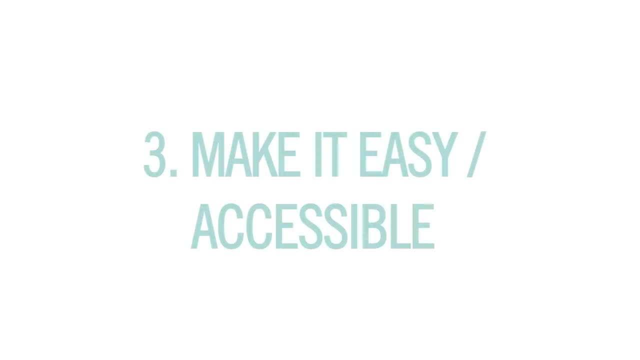 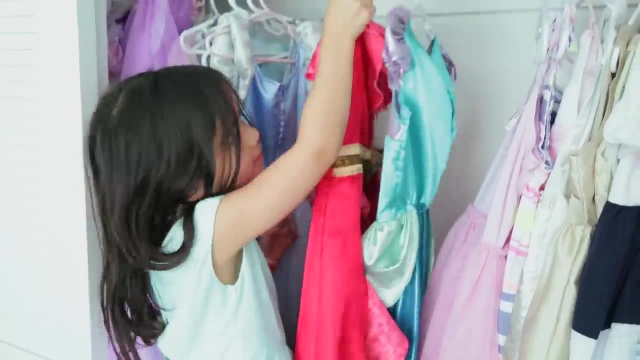 All done. We even decorated them. Number three: make it easy slash accessible. So this can be as simple as buying a step stool so they can actually reach to hang back up the play clothes that they could only rip down, or as in-depth as 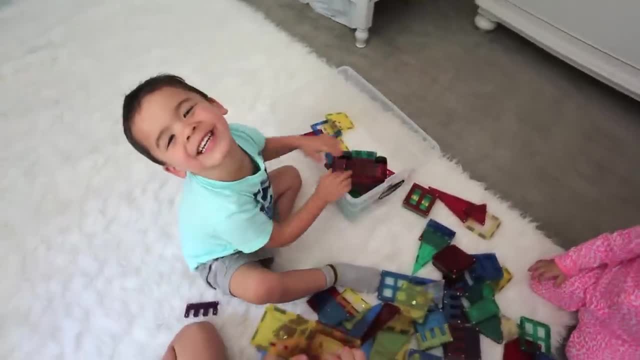 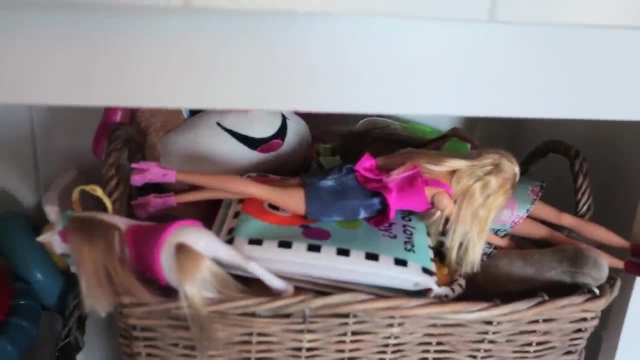 reorganizing their toys. I think that kids find it much easier to clean up when things are in clearly labeled individual items- Nice job, bunny- Rather than overstuffed containers. No, We are still working on that part of the house, But I truly love all of the. 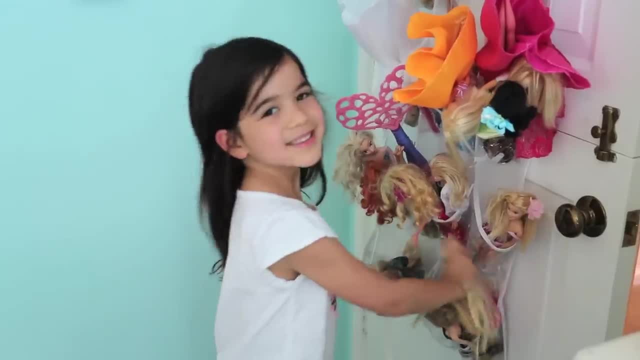 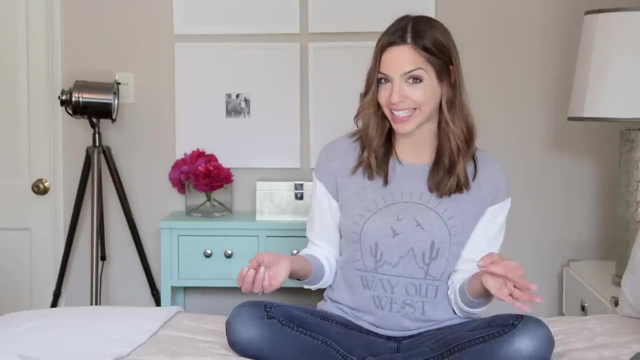 tricks we used in our mom hacks toy organization video, because they just make it so easy and fun for the kids. Number four find their motivation. So I just realized for Presley, this is play dates. Who's coming over today, Avery, Whether it's that day or the next week? 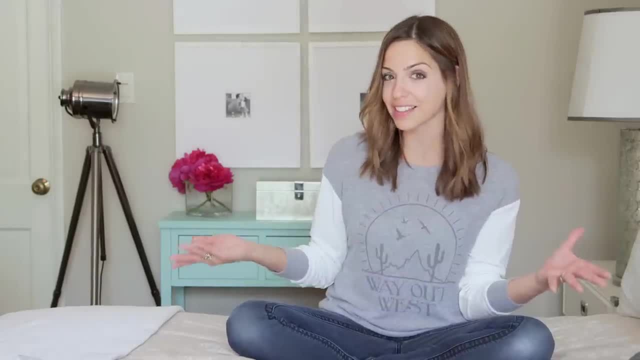 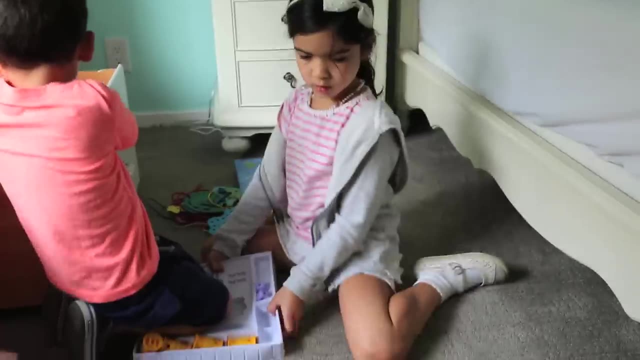 if I ask Presley: hey, do you want your friends to see your messy room like this? Number four must be no, because it really motivates her to get going. She is on a mission. We don't want it to be messy, right? 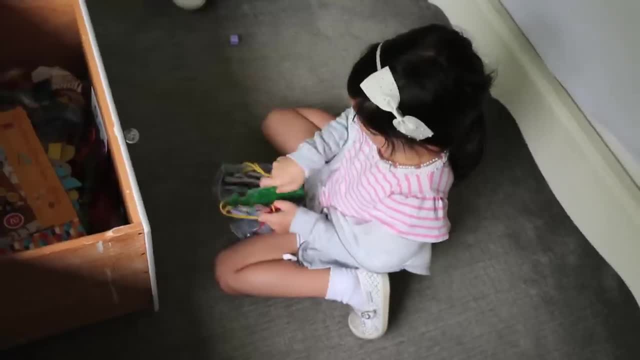 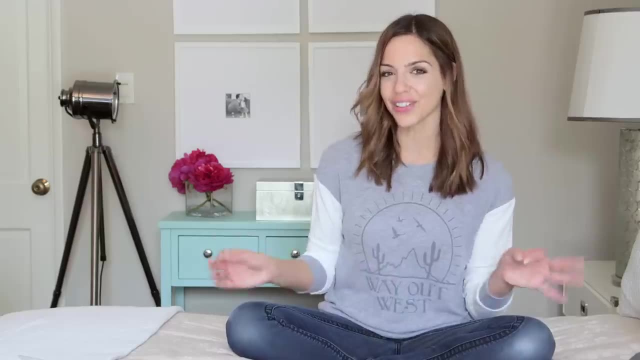 Yeah, Kids are also motivated by positive feedback. Oh my gosh, Presley, I'm so proud of you. Finally, number five, explain the much less attractive alternative. So if your compost go, like this Ford, it's time to clean up. No, And even begging does not work. 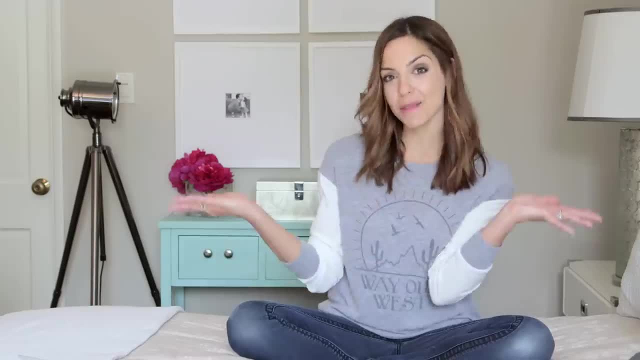 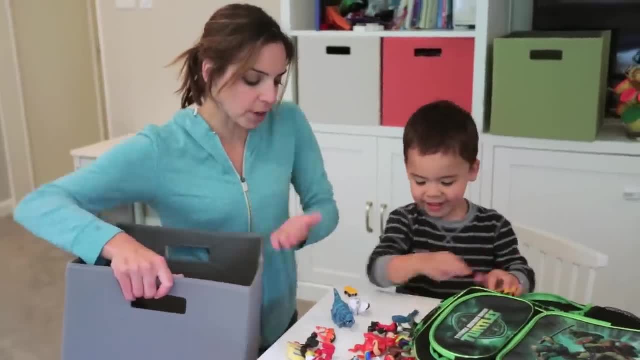 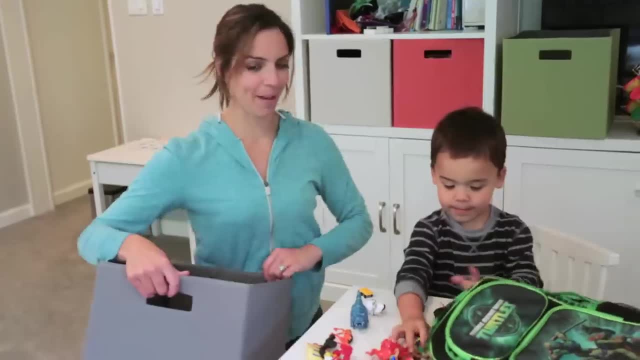 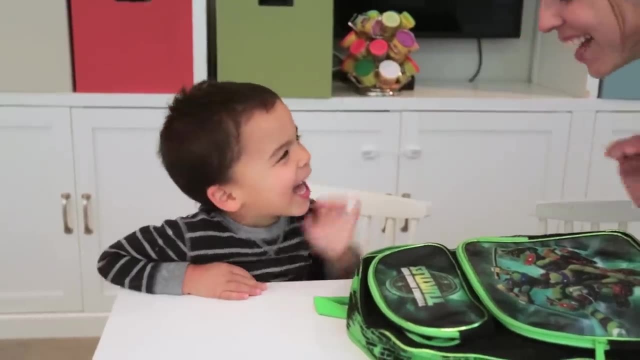 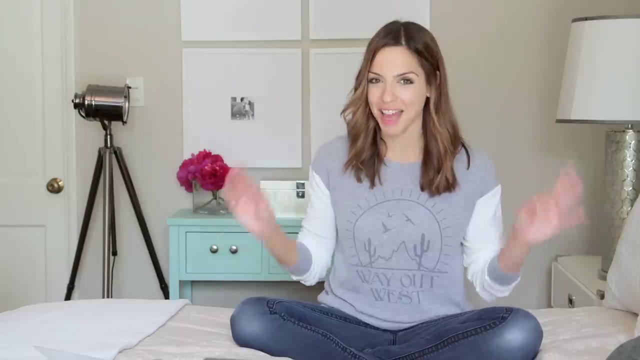 No in the basket. Okay, you're going to clean them up. Oh, now he's cleaned it up. This has had a really high success rate so far. High five, All right guys, we hope you find these useful and remember it is never too young to start, or at least attempt to have them. 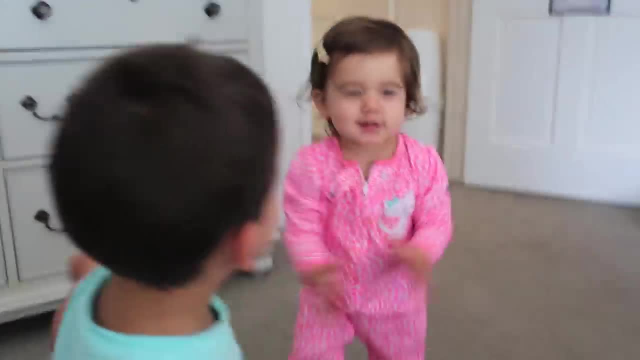 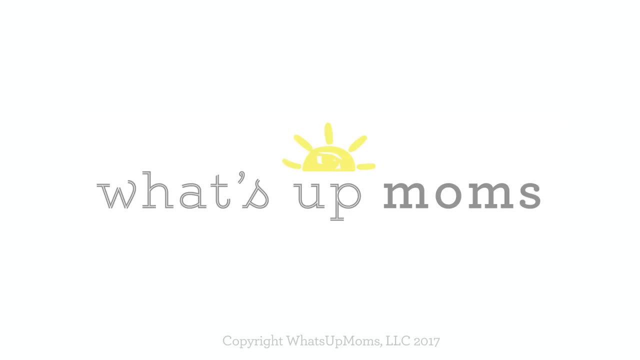 clean up. She's trying. Yay, Let me know what works for your family in the comments. I will see you next week week Bye.